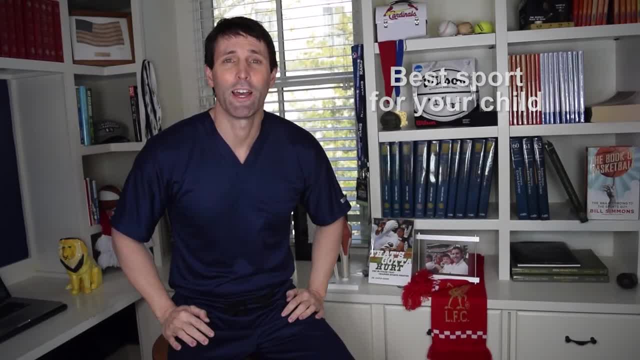 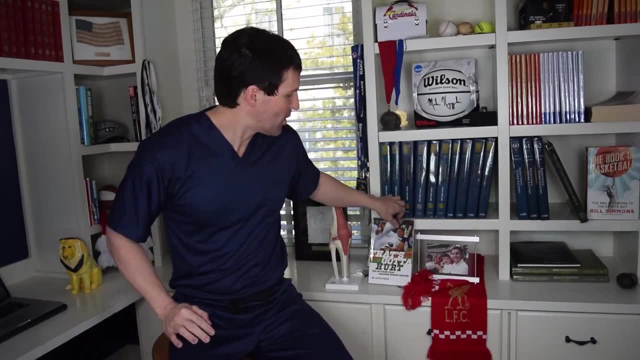 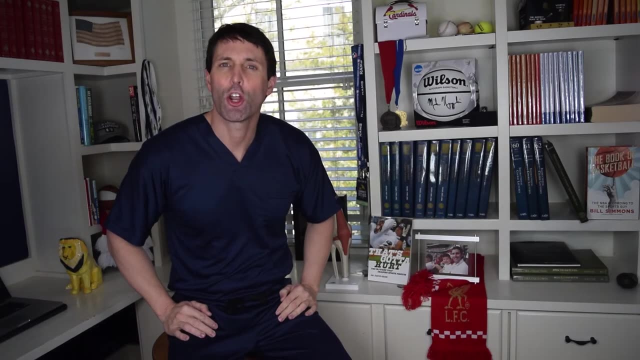 What's the best sport for your child to play? I'm Dr David, orthopedic surgeon, sports medicine specialist and author of the book That's Gotta Hurt- The Injuries That Change Sports Forever. I provide education, information and commentary on all sorts of sports and 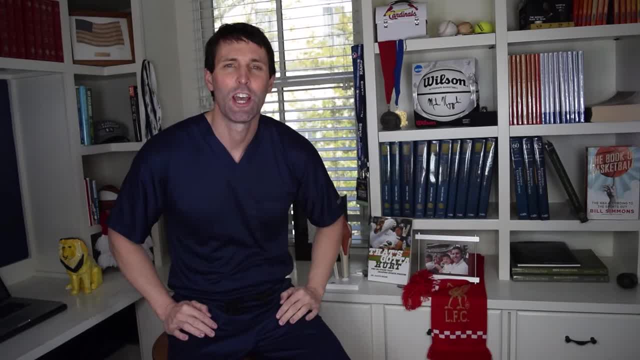 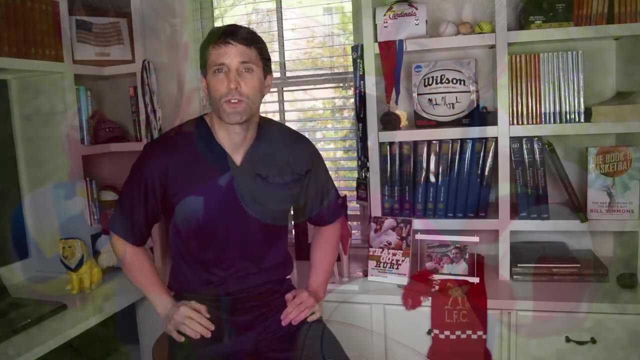 exercise injuries, injury treatments and injury prevention for athletes and active people, so that you can stay healthy and perform your best. I'm asked by a lot of parents what's the safest sport for their child to play. Now it's Youth Sport Safety Month, so this 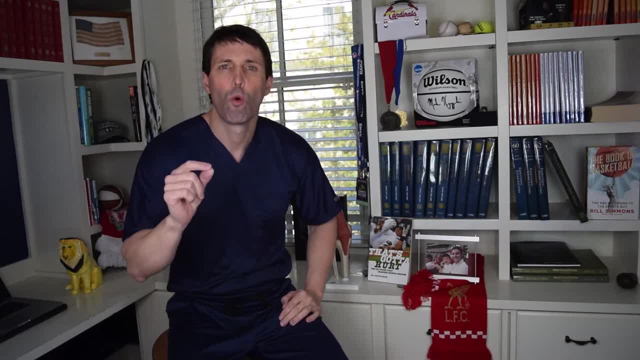 is an important topic, but I wouldn't really look at it as which one of the best sports there is to play, be it soccer or football or basketball or baseball, lacrosse, cheerleading, gymnastics, figure skating. I don't look at it that way. Here's what a lot of parents do: They have their child play one sport starting at a very early age. Maybe it's the sport that they played when they were kids and then they push their kids to play just that sport because that way they'll get better at it. They'll get chosen for the select club. teams or the travel teams, then maybe make the high school team and get seen by scouts and then get to the college level and the pro level. They push really hard in that one sport because they're afraid if they play different sports they're going to fall behind. But that's just not the case. Here's what I would do when you're letting your kids decide what sport they want to play, Starting at four or five or six. whenever they decide to start playing sports, pick one sport in that season and play it and see how it goes. 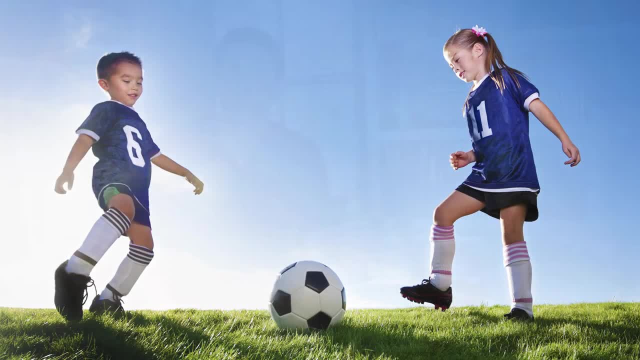 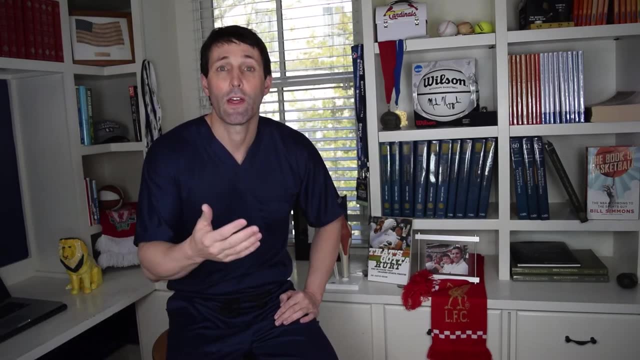 Then the next season, try a different sport, Then a different sport the season after that and let them try four or five different sports. That's what I did when I was a kid: Played soccer in the fall, basketball in the winter. 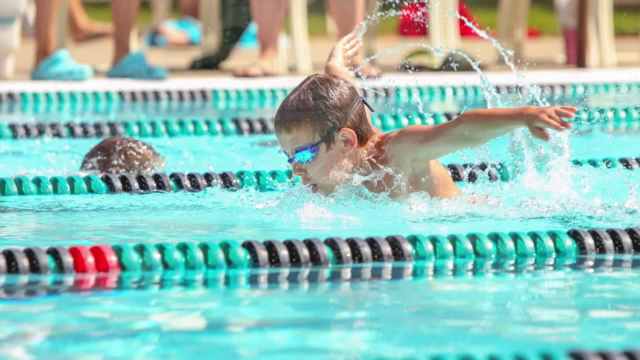 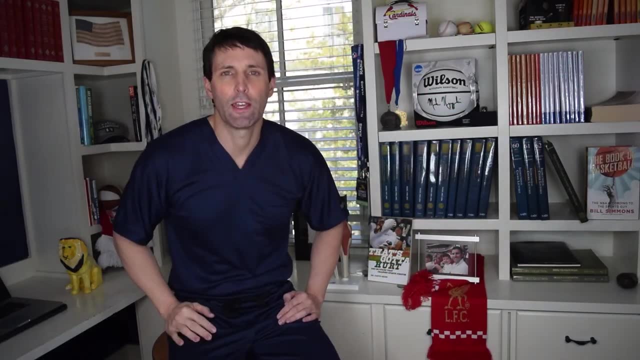 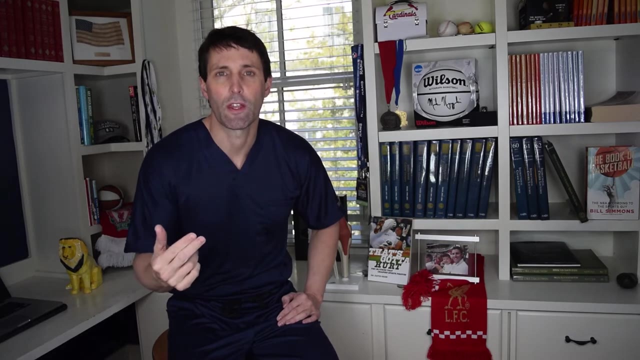 t-ball and baseball in the spring and swimming in the summer. I loved all of them, ultimately settled on soccer as I got older, And that's what I would want for your kids. Let them find the sport that they enjoy the most. Then they're more likely to stick with it. What you don't want is a situation where your child doesn't want to play soccer. You want them to get tired of a sport or burns out, Like 70% of kids in the United States who quit playing organized sports by age 13.. That's not what we want. We want them playing sports. 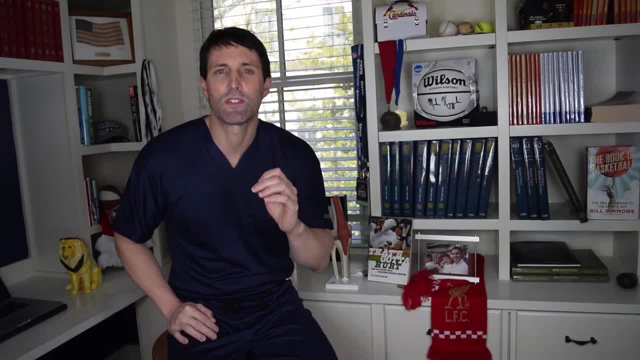 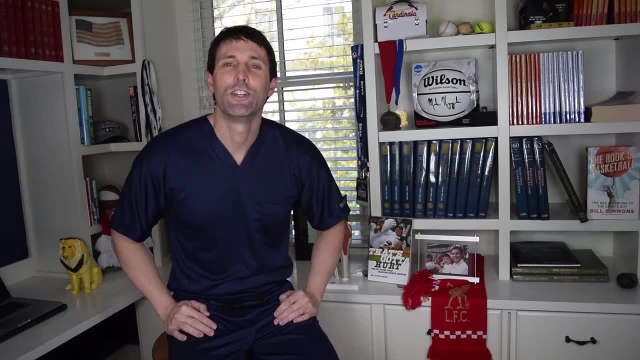 for so many reasons, but we need to let them stick with it, because it's the sport that they want to play, not the sport that you want them to play. Alright, do you have thoughts on how you pick the sport that's best for your child or in? 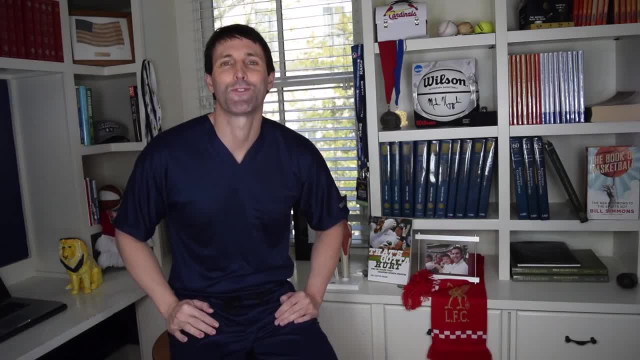 my words- how your child can pick the sport that's best for them. Let me know in the comments. I would love to hear what you have to say If you like videos like this and you want more information on sports and exercise injuries, injury treatments and injury prevention.